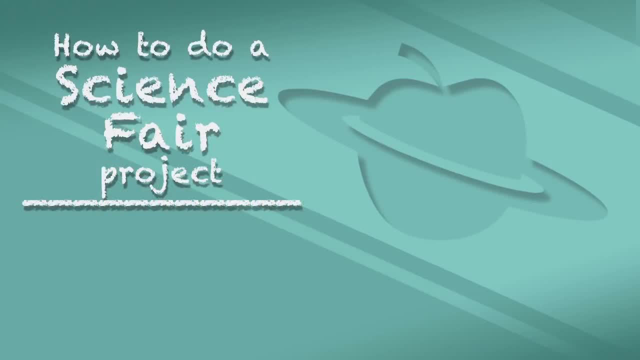 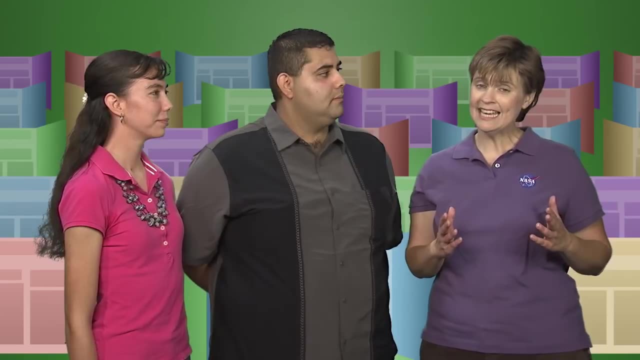 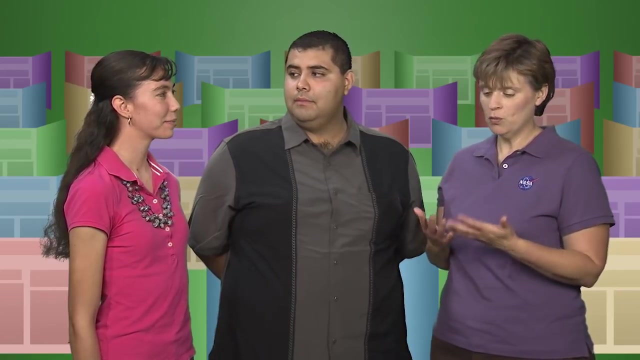 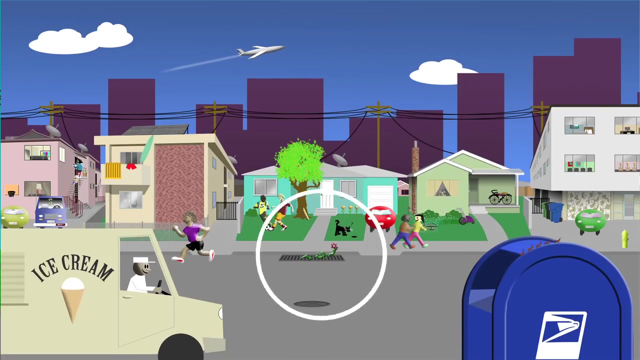 Now it's time to develop your idea into a testable question. Serena, you had several really good ideas from our image. Can you pick one of those and lead us through how you might develop that into a testable question? Looking at the picture, I'd seen the plant growing out of the storm drain. 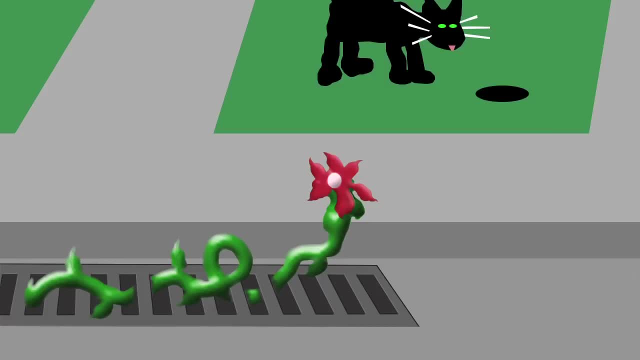 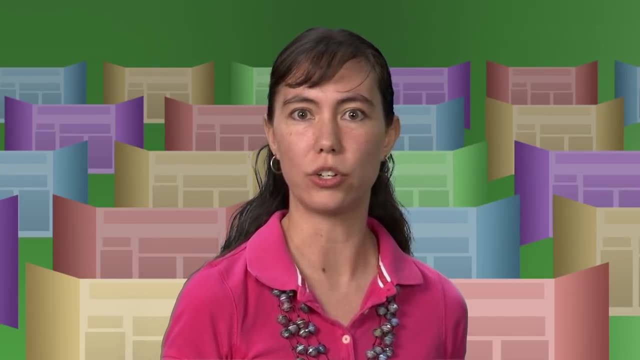 and that might lead to questions of how do plants grow, under what conditions do they grow best? And so you want to just pick one idea, one thing to test. so I might restrict my question to how much dirt does a plant need to grow? 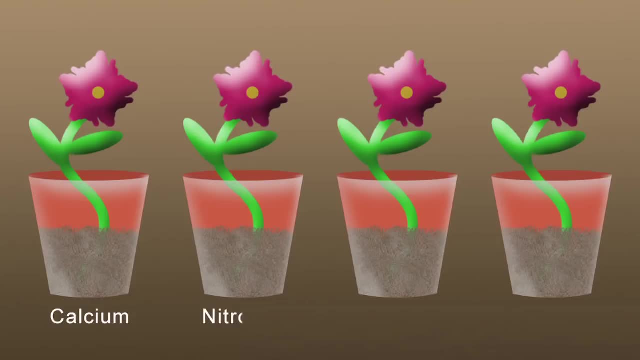 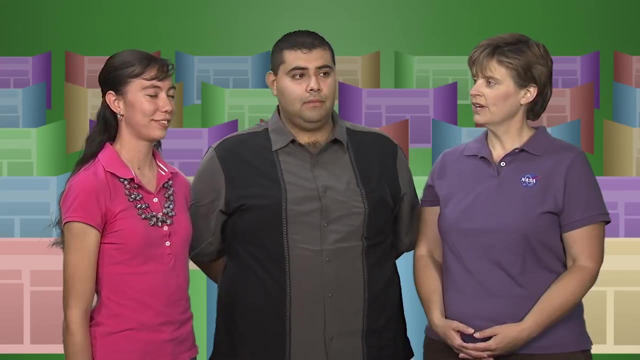 Or you could decide instead to test different fertilizers, but you want to pick one bite-sized science question and then use that to set up your science investigation. Okay, so you might be able to vary the amount of dirt, and we would want to keep track of the amount of dirt. 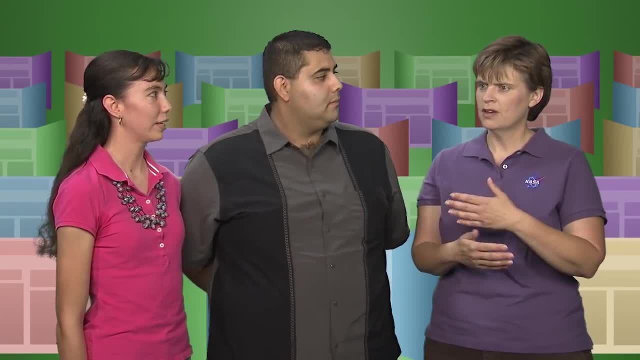 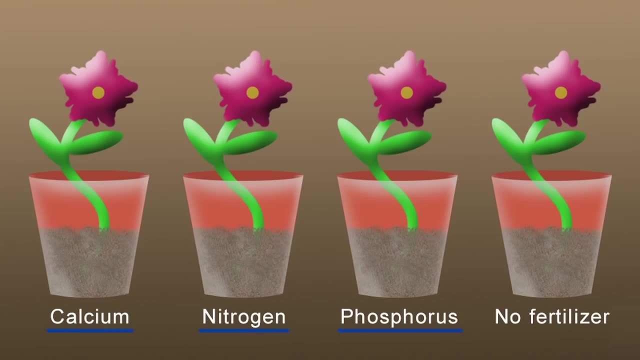 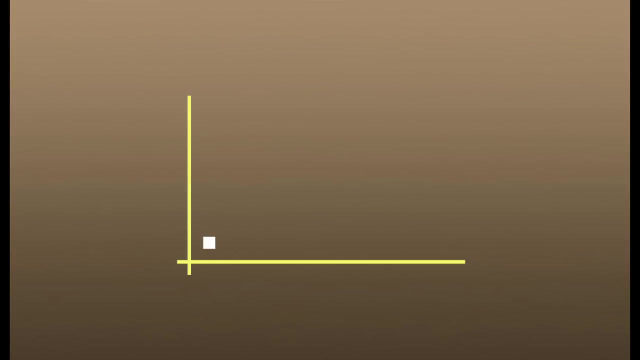 or the different types of fertilizers. How many types of fertilizers might you try? Generally, you want to experiment with probably at least three different options for each one. It'll, of course, depend on your science question, but if you just have one data point, of course that doesn't really tell you anything. 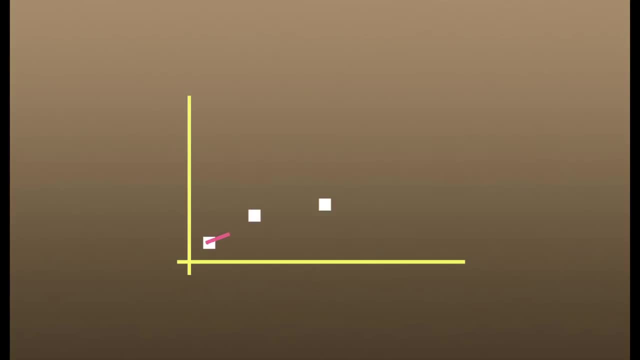 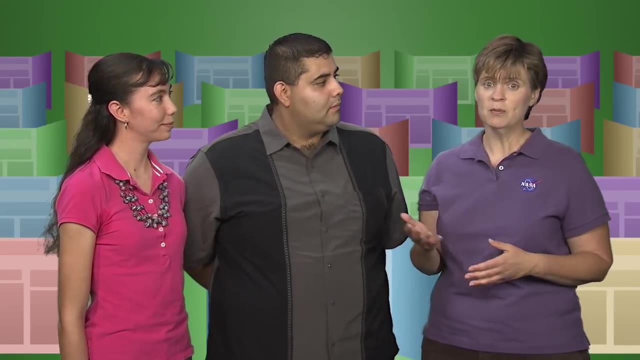 You need two to compare and then three to really start seeing a trend, and then obviously more if possible is usually better. Okay, so you'll want to be sure to measure your results somehow. Measuring the results on a plant might involve. 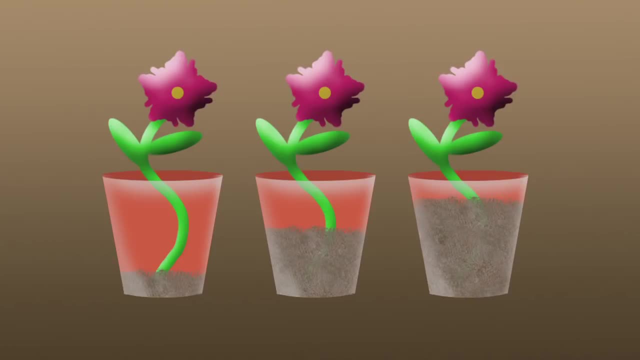 It just depends on what you're measuring. If you're looking for the health of the plant, you could look at plant height. If it's a blooming plant, how many flowers perhaps come out? You could look at its root system, perhaps. 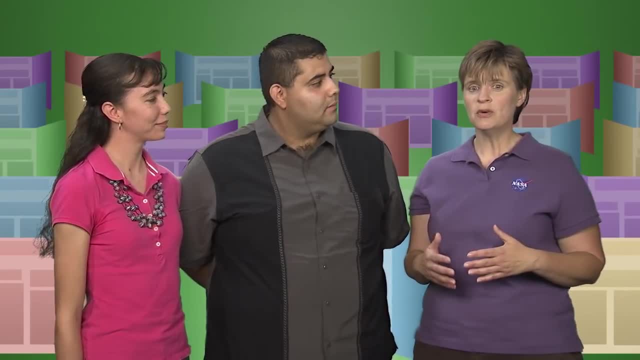 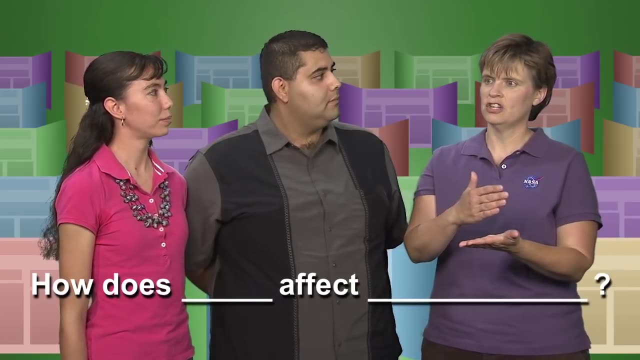 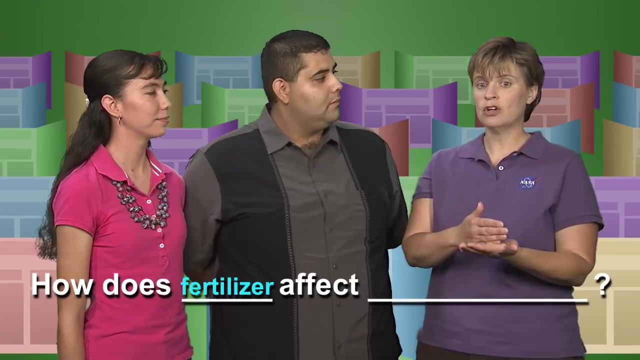 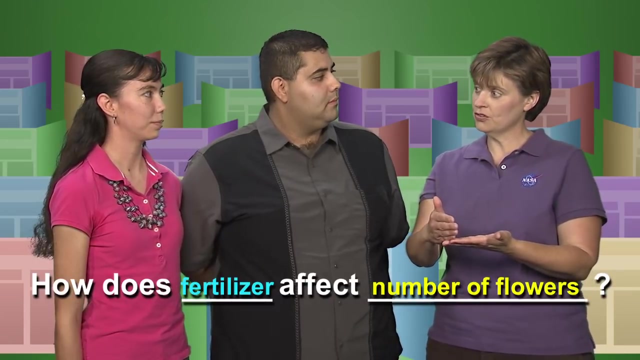 It just depends on what you're measuring. Okay, so the question would be something along the lines of how does this affect this And your? this and this would have to be specified very clearly so that you would be measuring either how does fertilizer affect plant growth in height, or how does fertilizer affect number of flowers. 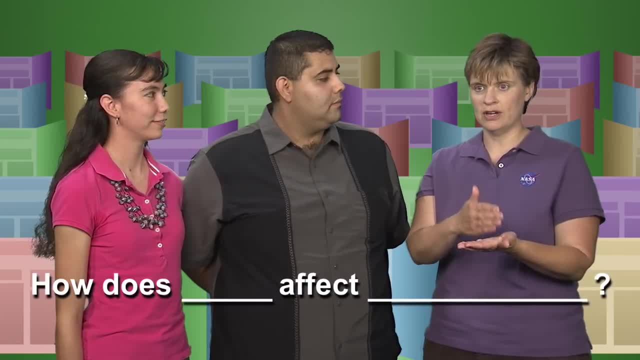 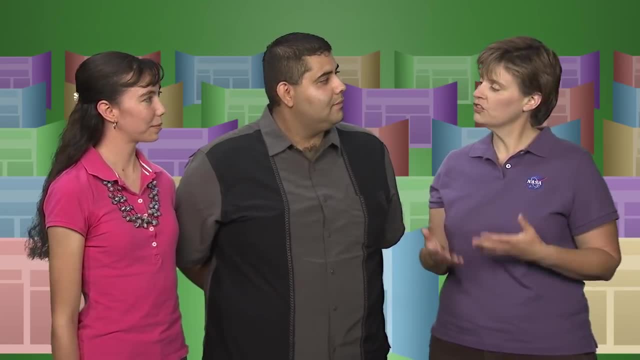 So you would need to make sure that you specify your input variable and your output expectation. Okay, so, Arby, tell me about one of the things you saw in this image that you could ask a question about, and what your development of that question would entail.